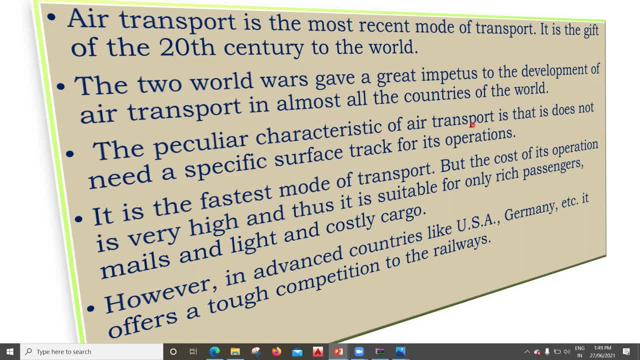 Only the landing and all is required, But you don't require a Track like we have it for the railways. Next point is: it is the fastest mode of transportation, but the cost of its operation is very high, And thus it's suitable for only rich passengers and mostly for the cargo. 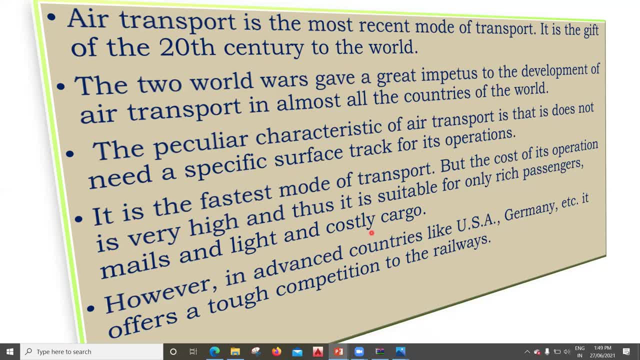 But nowadays, if you look the airport, I mean, the flight can be taken by any people. Few years back the tickets were expensive, but now it's not that expensive, So we cannot say that only rich people can take this. 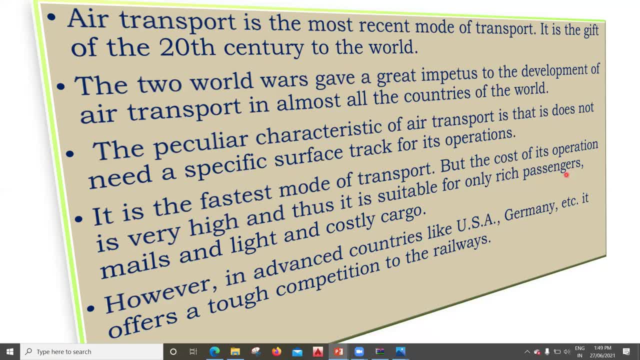 Almost all of All of them can take this, that is, air transportation can be taken by all sorts of people in the society. And the last is, however, in the advanced countries like USA, Germany, etc. it offers a tough competition to the railways, right. 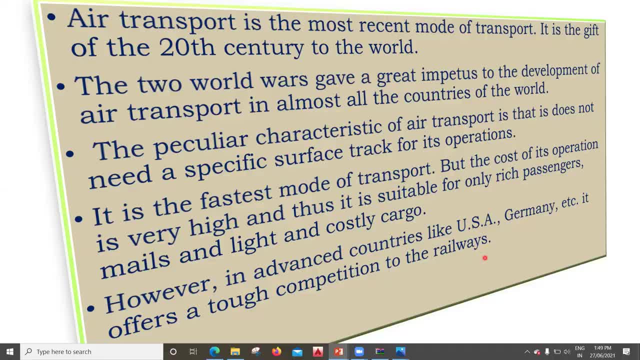 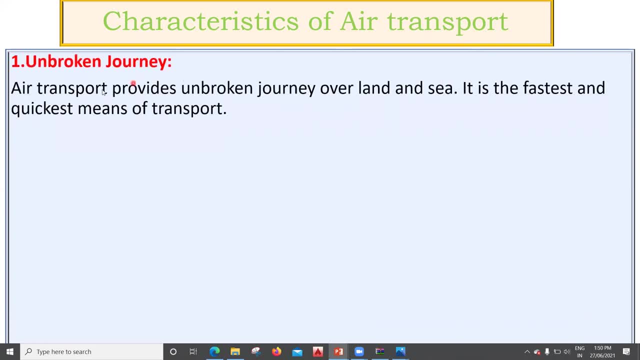 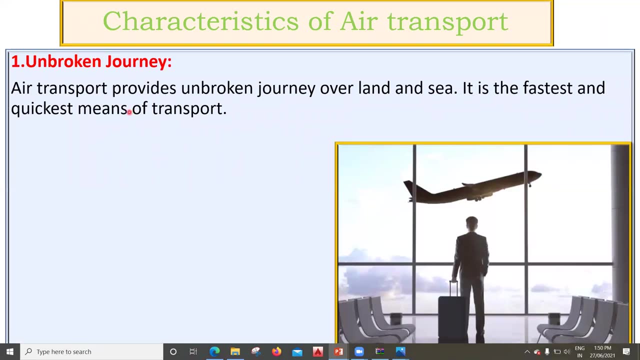 So this is a bit theory, what we need to understand about the airport. Yeah, Now coming to the characteristics of the air transport. The first is the unbroken journey. Air transportation provides unbroken journey Over the land and the sea. it is the fastest and the quickest means of transportation. 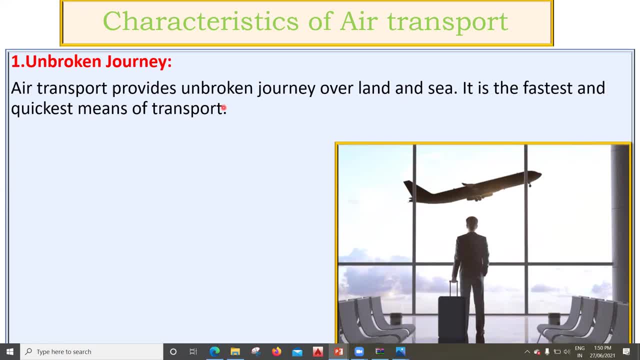 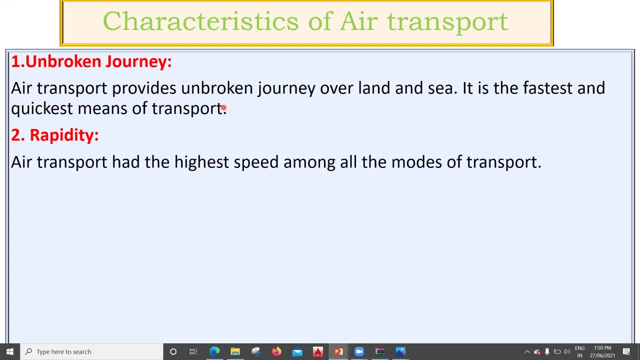 When compared to all other airport air transportation is the fastest and the quickest mode of transportation. Next is rapidity: Air transport has the highest speed among all the modes of transportation, and we know that. Third is expensive: Air transport is the most expensive means of transportation. 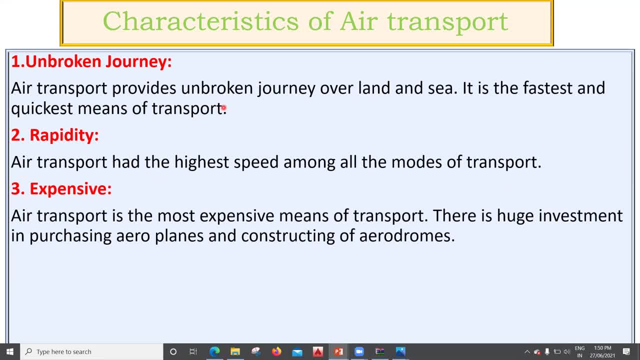 There's a huge investment in purchasing the airplanes and also the constructing of the aerodromes right. It requires a huge investment if you want to set up an airport And also a huge investment is required in purchasing the aeroplane. 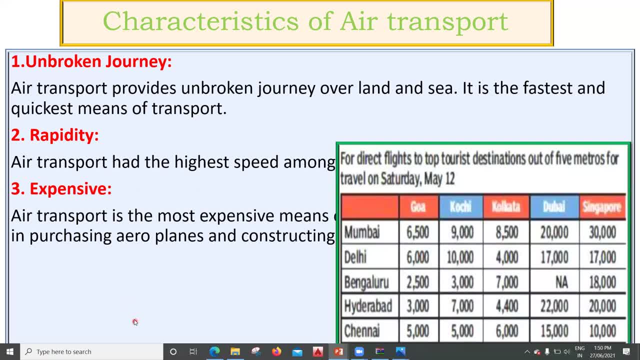 So the next one is that, yeah, these are the few flight tickets, The rate of the flights, what I put here: if you want to go from Mumbai to Goa, it's 6500 rupees, From Mumbai to Kochi, it is 9000 rupees, and so on. right. 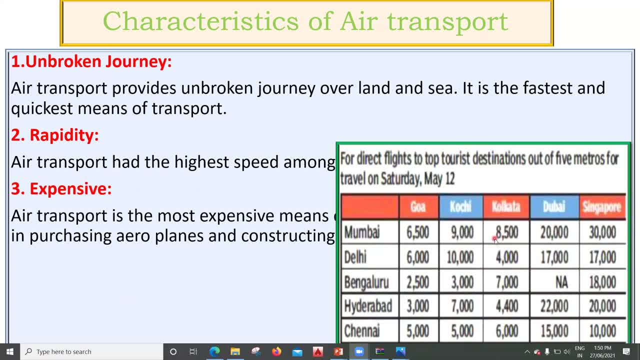 These are the normal rates, usually what we get, But they keep on fluctuating depending on the day and also depending on the flight time. So this is a good thing. Which company flight you're taking up? yeah, And the next one is special preparation. 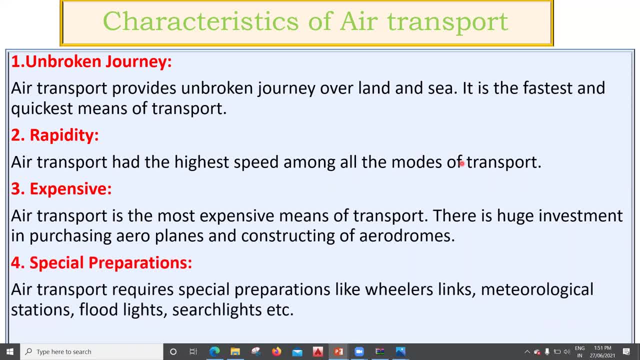 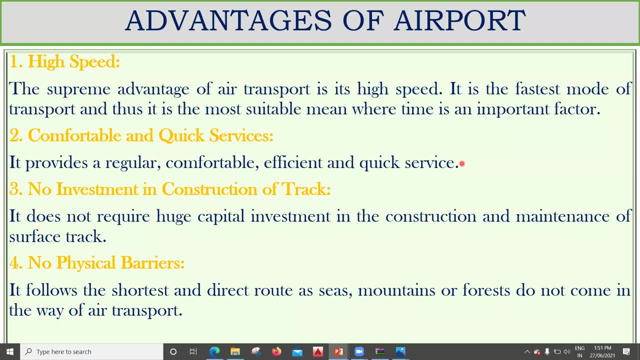 Air transport requires special preparation, like wheeler sling, the meteorological station, floodlights, surge lights and etc. So again, the special preparations is required here. Next, coming to the advantages of the airport. First one is high speed. 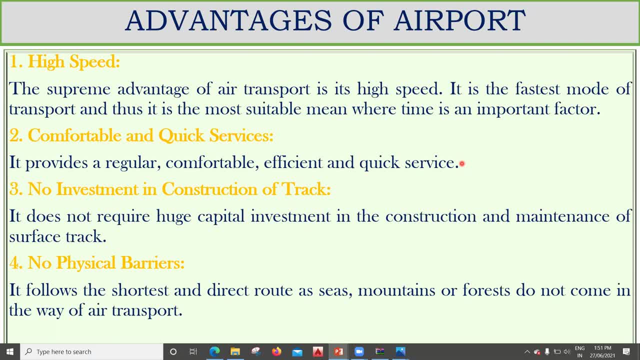 The supreme advantage of air transport is it's a high speed. It's the fastest mode of transportation And thus it is most suitable, I mean when That's the base of all the services. But the travel time is the important factor. 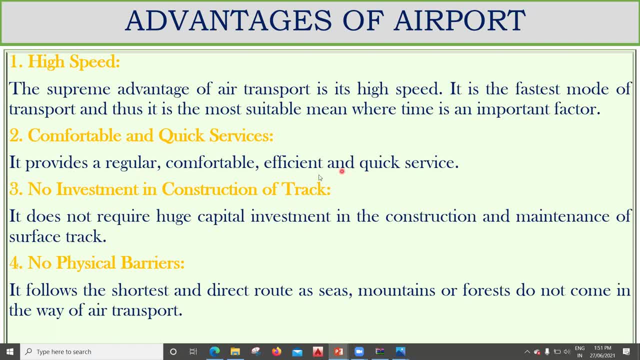 Next is comfortable and quick service. It provides a regular, comfortable, efficient and quick service. Next third one is no investment in the construction of the track, which you already seen. It does not require a huge capital investment in the construction and the maintenance of the surface track. 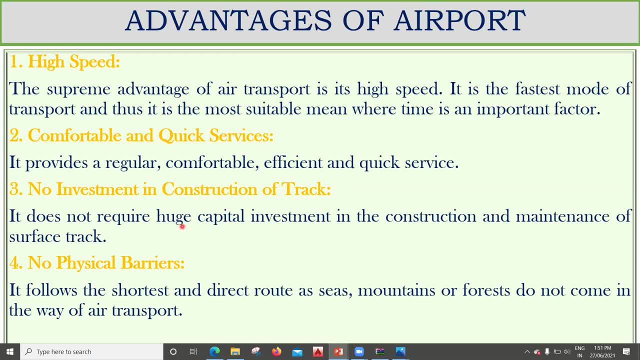 Unlike in the railway, we need to do regular maintenance and all. But whereas in case of airport and all, there is no track has such of course there will be runway and all. so that can. that comes under the different part and there also regular maintenance has to be done. next is no physical barriers. it follows the shortest and 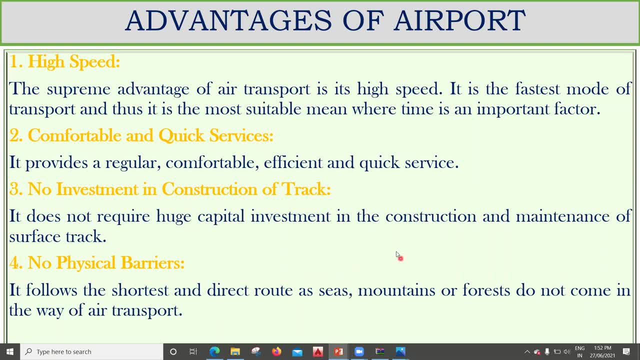 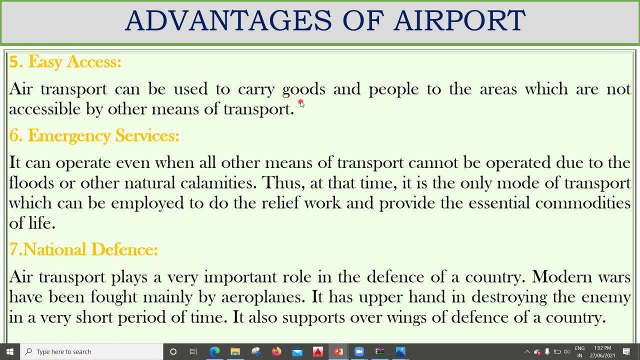 the direct route has. these mountains or forests do not come in the way of a transportation, right. yeah, so next is easy access. a transportation can be used to carry goods and people to the areas which are not accessible by other means of transportation. right, especially if you go to the 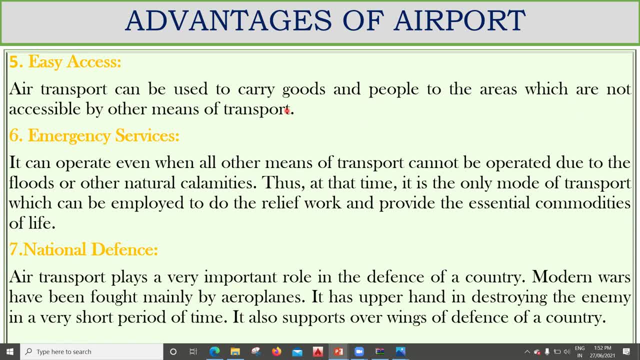 hilly areas and all where the railway transportation is very difficult. in that case, air transportation will help us a lot. yeah, the next is emergency services. it can operate even when all other means of transportation cannot be operated due to the floods or other natural calamities. thus, at that time, it is only mode of transportation which can be employed to do the 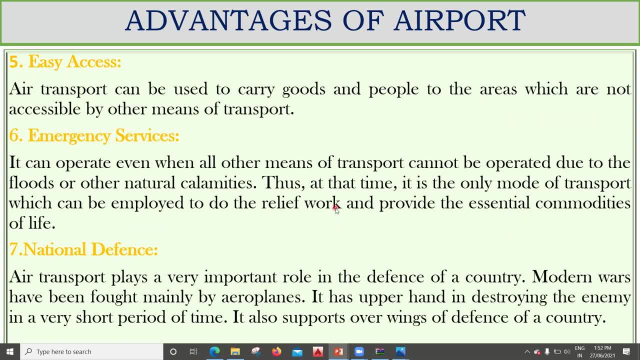 relief work and provide essential commodities to the life. we also seen this during the floods and all especially in the north, north, northern, north eastern part of india and all. so whenever there is a flood and all we always have seen the national uh disaster team. they come with the 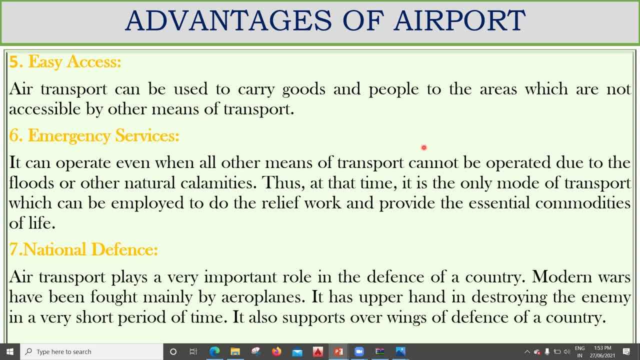 helicopter and they give the all the necessary things that is required. so air transportation will help us in terms of floods and all where we cannot, you know, take the rail with help. we cannot make use of railway or other mode of transportation during this time. okay, now next is in the national defense. air transport plays a very important role in 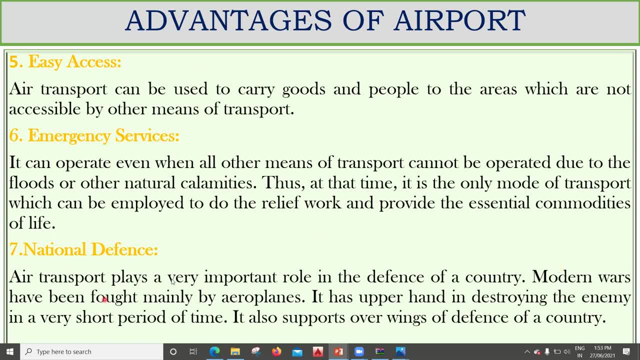 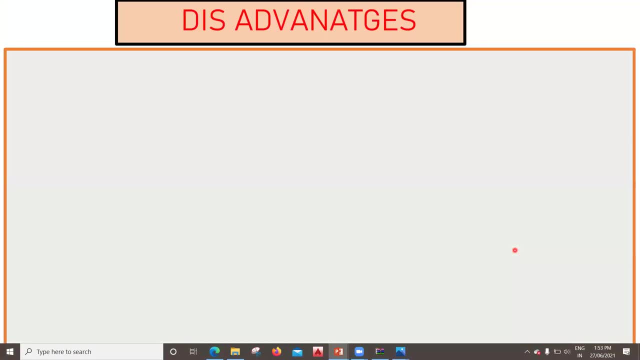 the defense of a country. modern world wars have been fought mainly by aeroplanes. it has an upper hand in destroying the enemy in a very short period of time and it also supports our wings of defense of the country. we also have seen that we are lots of fighter jet. aircrafts and all so also it helps in the national defense for the security of our country. yeah, now coming to the disadvantages first, is very costly. we already seen that it is the costliest means of products creation. such, if you are using the, become necessary technological defense. what you can say about these air transport and that'll be in our development and uses at 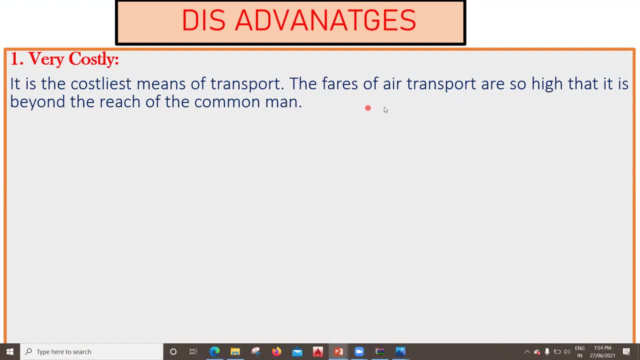 costly. we already seen that it is a costliest means of transport. the fees of a transport are so high that it is beyond the reach of a common man. but, as i mentioned, uh, as of as of now we can travel with the flight. it's not that expensive also. yeah, next is small carrying capacity. its 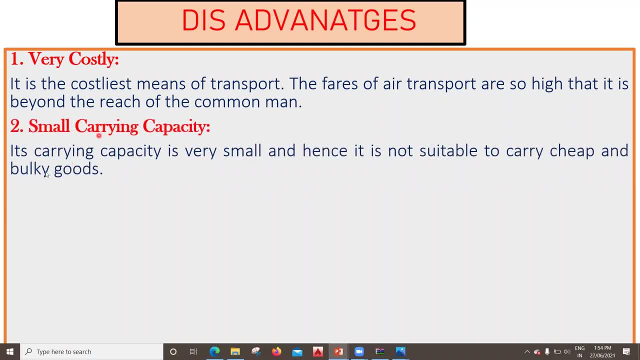 carrying capacity is very small. hence it is not suitable to carry cheap and bulky goods. right, because if you have seen a average normal flight, they can carry up to 300 to 350 passengers, but if you try to travel through a rail sandal, it can carry more than a thousand, five thousand and 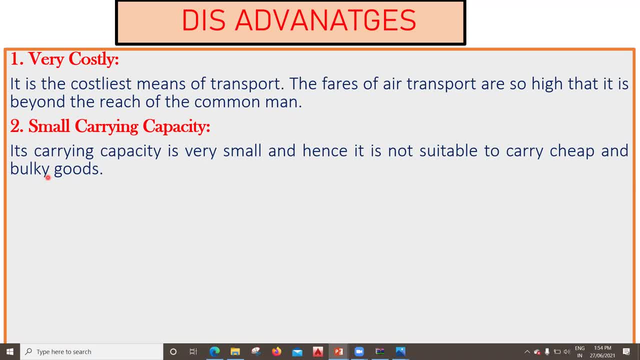 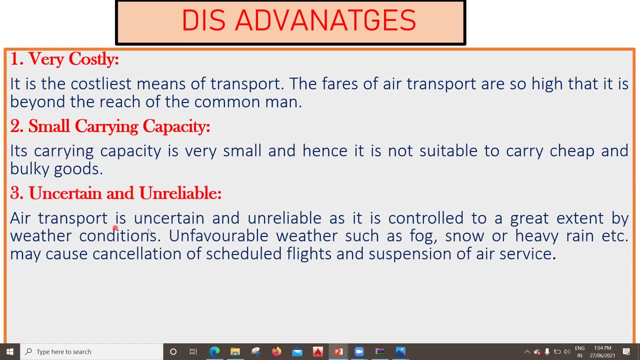 more than thousand passengers at once, right. so that is why, in comparison to the railway transportation, it has small carrying capacity. next is uncertain and unreliable. air transport is uncertain and unreliable as it is controlled to a great extent by the weather capacity. it is not suitable to carry heavy goods. it is not suitable to carry heavy goods. 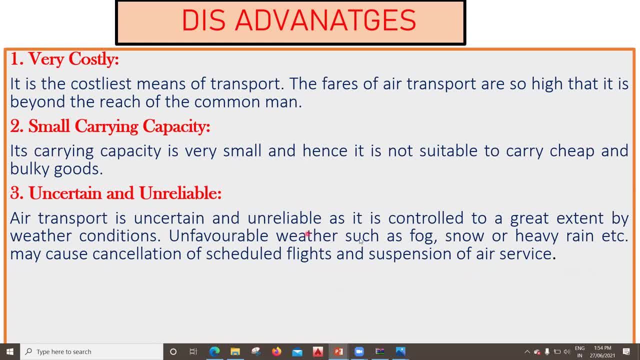 conditions, because everything depends on the weather condition. unfavorable weather, such as fog, snow or heavy rain, etc. may cause cancellation of the scheduled flights and suspension of the air services, especially in the month of october, november, december, when there is a, you know, heavy rain and all, and also during the winter season becomes very difficult for the operation of the. 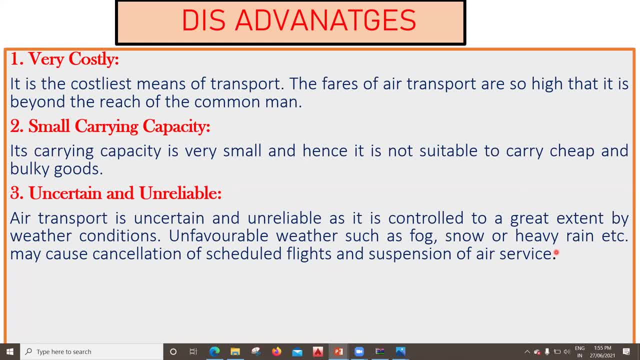 aircraft, so sometimes it will create a problem, so that is why it is uncertain and unreliable. next is breakdown and accidents. the chances of breakdown and accidents are high as compared to other modes of transportation, hence it involves a comparatively greater risk. yeah, see, risk is everywhere, even if you transport. 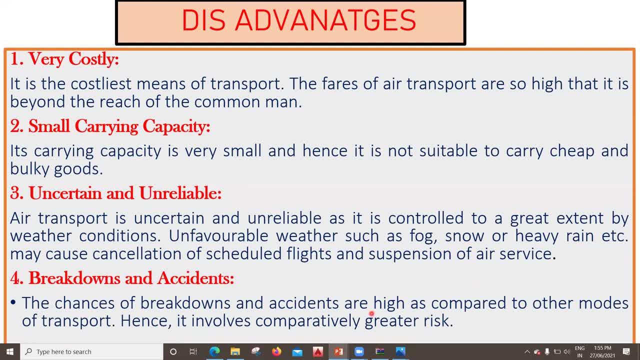 even if you travel by uh rail also, sometimes there are chances that you will meet, meet up with the accident and all, but in comparison to the other mode of transportation, every time you take off you will be having a fear in you and all, and also whenever you do the landing, there will be fear in. 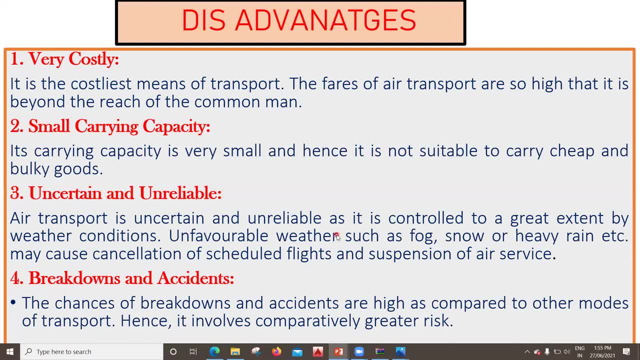 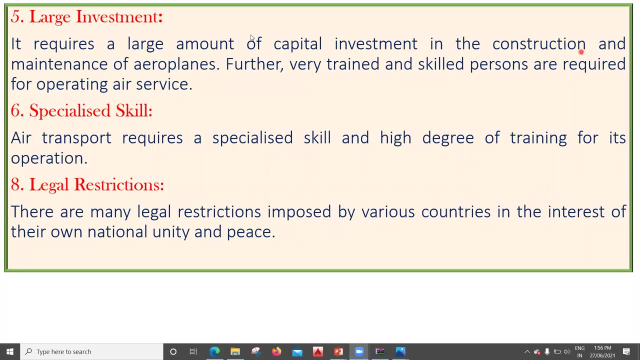 you when compared to other mode mode. of course, in air air transportation the probability of risk is little more in comparison to the other modes of transportation. next is large investment. it requires a large amount of capital investment in the construction and maintenance of the airplanes. further, very trained and skilled. 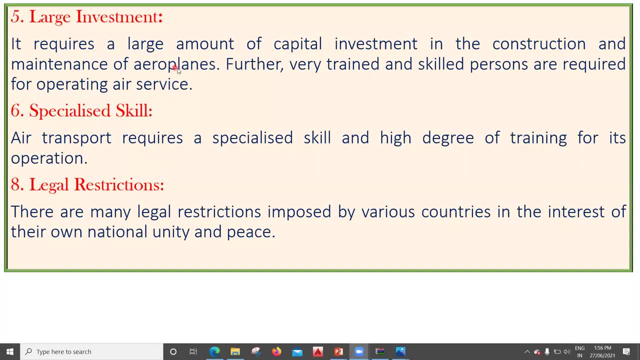 persons are also required for operating the air services right, so we require a very skilled persons. we have airport authority of india which conducts exams for all this post, for the air traffic controller and all, and then, once you clear the exams and all, you'll be given a training. so 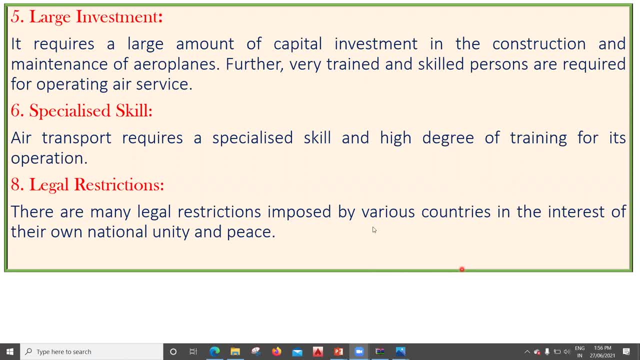 once you pass the training, only then they are going to take you for the job. so it requires a lot of skilled persons and also proper training. next is specialized skill. air transport requires a specialized skill and high degree of training for its operation. the pilots also how to undergo. 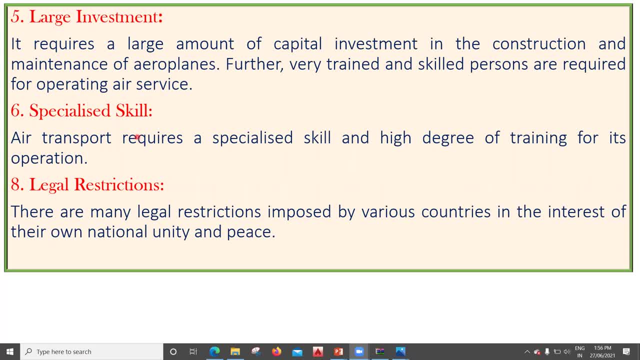 training right, so that is a very skilled person. so we have airport authority of india which conducts exams for all this way. it's written specialized skill and the last is a legal restrictions. there are many legal restrictions imposed by various countries in the interest of their own national unit and peace. 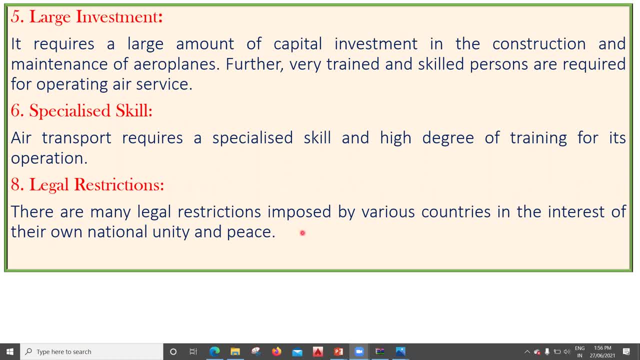 right, so you cannot go in any country without the permission. you have to take permission from the other country so that you can do very smooth landing and take off in different countries. prior. prior to doing this, we need to take permission from them, right? yeah, so all this was about the 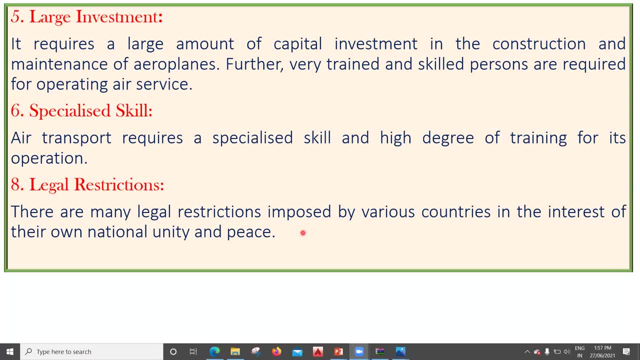 advantages, the disadvantages and the characteristics of the aircraft or the airport. so in the next lecture we'll try to see other things, how the classification of the airport is done and all those things. so we'll see you back in the next lecture, thank you.